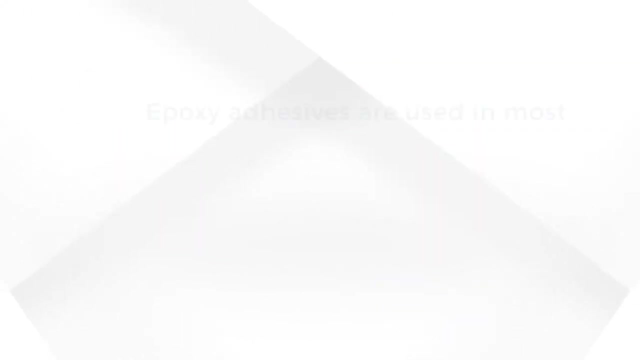 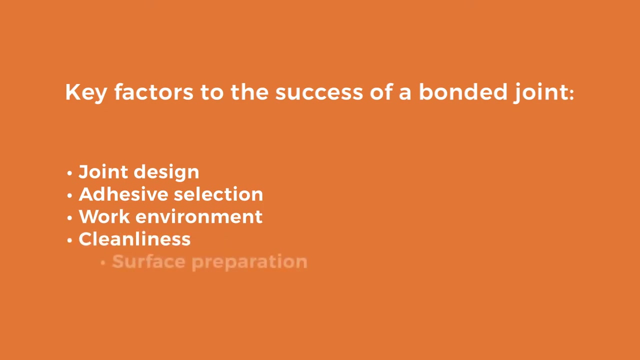 and urethane Epoxy adhesives are used in most aerospace applications. Adhesives are generally available in the form of paste or film. Key factors to the success of a bonded joint: Joint: design, adhesive selection, work environment cleanliness, surface preparation, tooling and fixturing, bonded process, workmanship, quality assurance and non-destructive inspection. 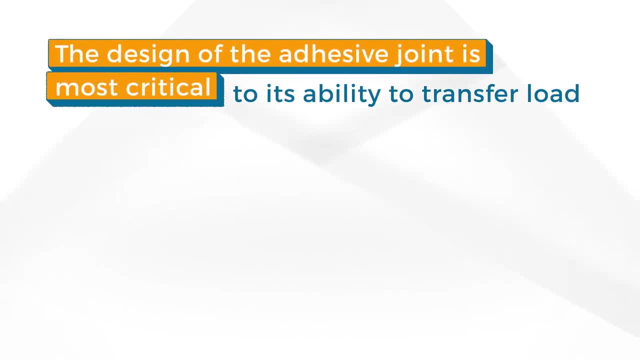 The design of the adhesive joint is most critical to its ability to transfer load. Adhesives perform best in shear, not tension or peel. Bond areas should be sufficient so that stresses do not exceed allowables. Geometry-included stress concentrations can significantly reduce the load-carrying capability. 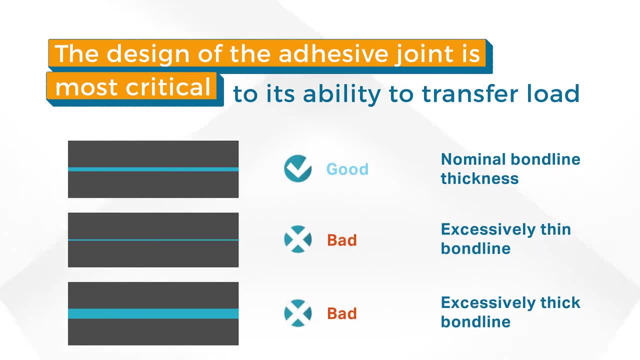 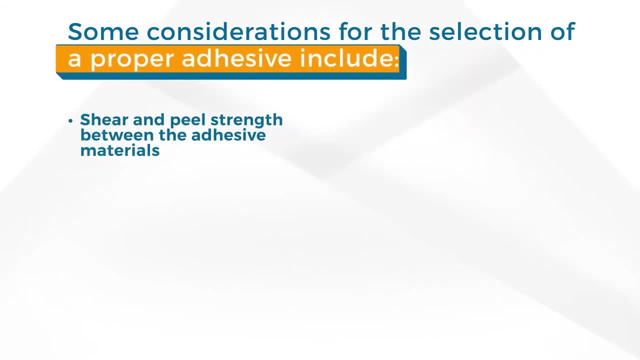 Excessively thin or thick bond joints carry less load. Some considerations for the selection of a proper adhesive include Shear and peel strength between the adhesive materials. creep, fatigue, elongation or brittleness. viscosity to ensure the adhesives stay in place. 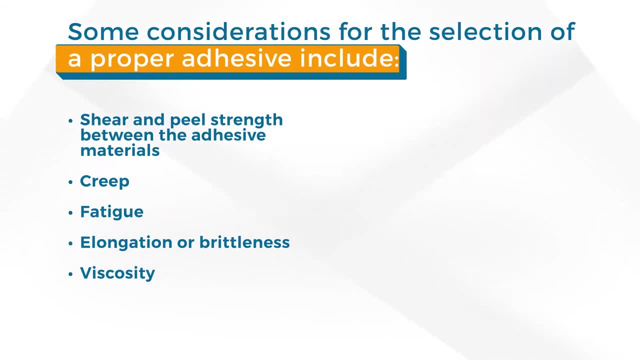 fills the joint and wets to the bond surfaces. Compatibility with adherence and surface preparation procedures. Pot life, to ensure that adhesives do not begin curing before the assembly is complete. Shelf life and out time. Temperature resistance, to ensure the joint does not fail due to excessive heat or cold. 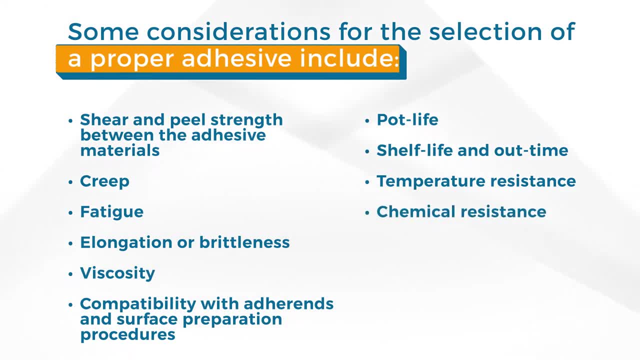 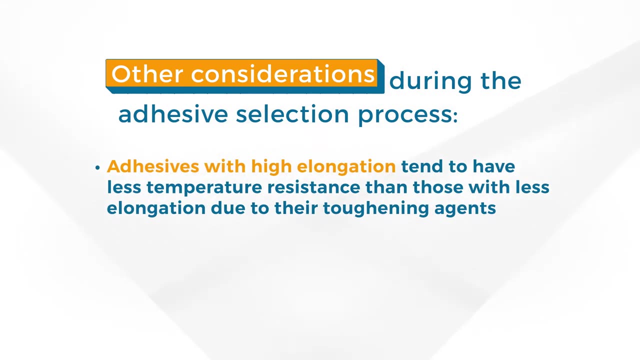 Chemical resistance to ensure adhesives do not degrade by the chemical exposure. expected Cure requirements including time, temperature and pressure. the adhesive is compatible with the bonding process. Other considerations during the adhesive selection process: Adhesives with high elongation tend to have less temperature resistant than those 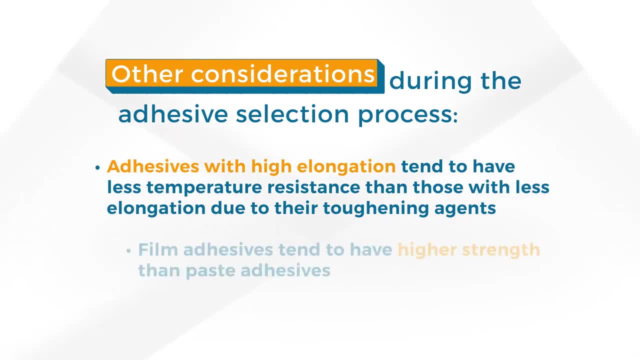 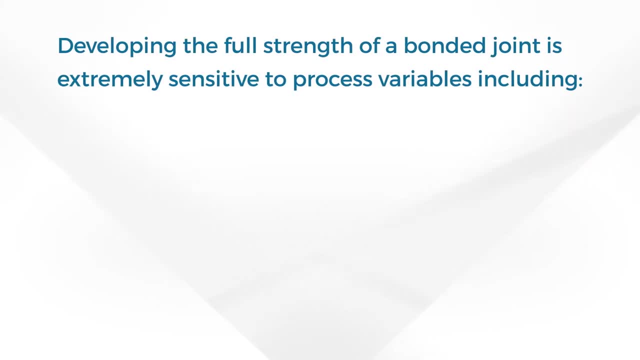 with less elongation. due to their toughening agents, Film adhesives tend to have higher strength than paste adhesives. Developing the full strength of a bonded joint is extremely sensitive to process variables, including surface preparation pre-bond moisture in the adherence. 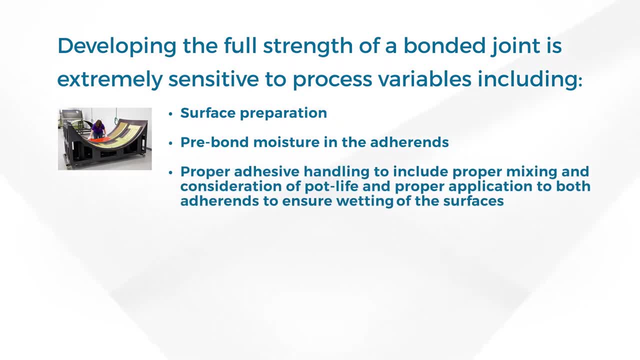 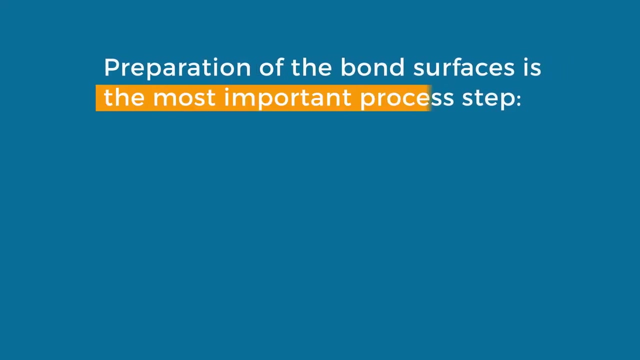 proper adhesive handling to include proper mixing and consideration of pot life, and proper application to both adherents to ensure wetting of the surfaces. Application of correct pressure during cure to ensure full contact and eliminate voids. bond line thickness control. proper cure time, temperature and temperature ramp rates. Preparation of bond surfaces is the 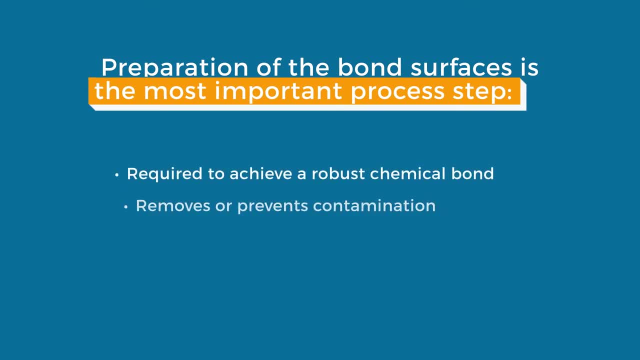 most important process step Required to achieve a robust chemical bond. removes or prevents contamination. creates chemically active sites on the surface. Many aerospace metals require a chemical etch or adhesion promoting layer and a primer or other coating for ultimate strength and bond durability. Common composites and polymer surface preparation methods include: 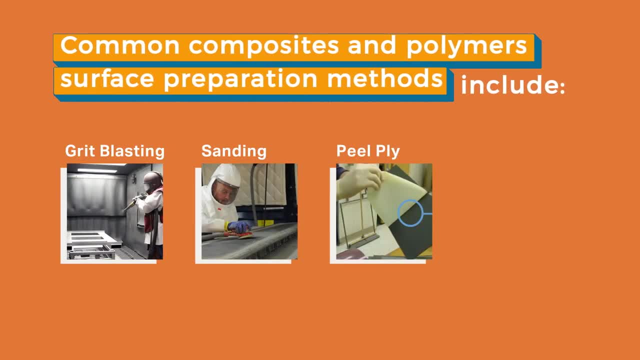 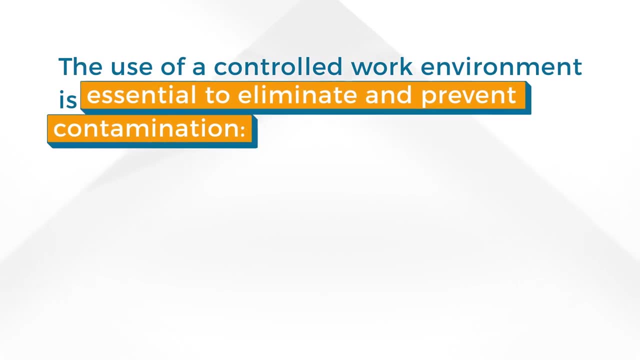 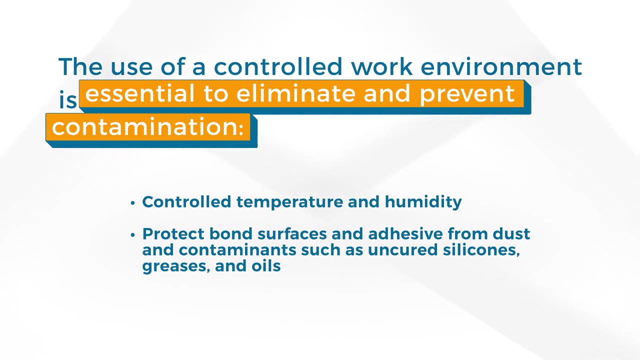 grit, blasting, abrasion and sanding peel, ply and energetic. The use of a controlled work environment is essential to eliminate and prevent. Controlled temperature and humidity can affect adhesive pot life, viscosity, moisture uptake in the adhered surface, formation of voids in the bond line, amine blush formation and cure. 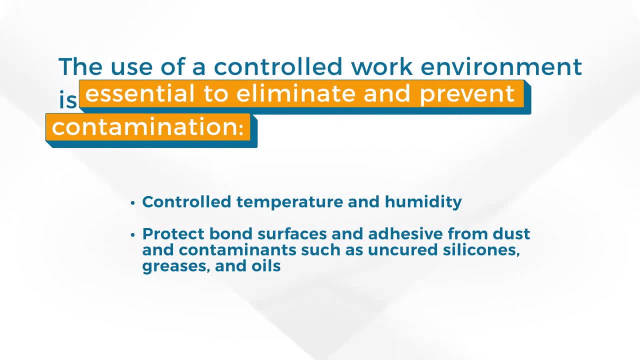 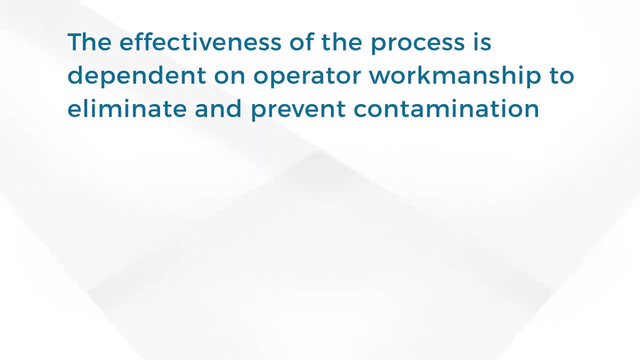 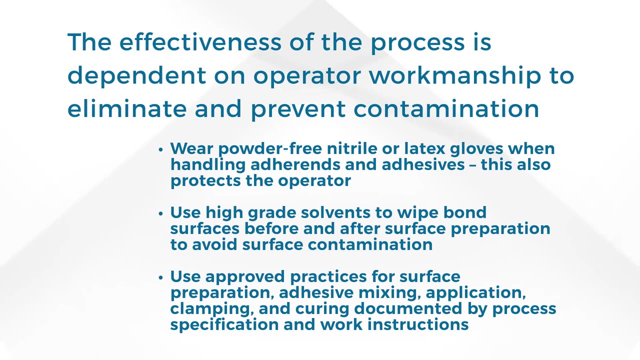 Protect bond surfaces and adhesive from dust and contaminants such as uncured silicones, greases and oils. The effectiveness of the process is dependent on operator workmanship. to eliminate and prevent contamination, Wear powder-free, nitrile or latex gloves when handling adherents and adhesives. This also protects the operator. 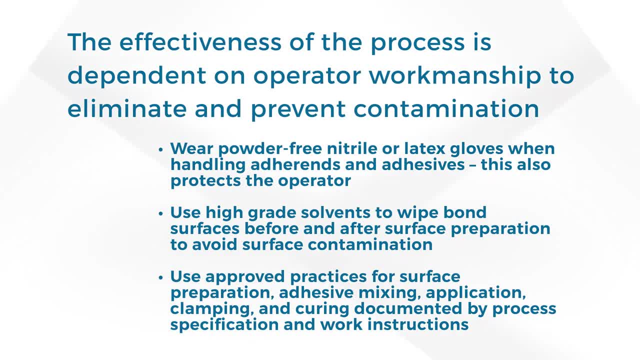 Use high-grade solvents to wipe bond surfaces before and after surface preparation to avoid surface contamination. Use approved practices for surface preparation, adhesive mixing, application, clamping and curing, documented by process specification and work instructions. Quality Assurance: Visual inspection of bonded assemblies is performed to look for the best possible quality. 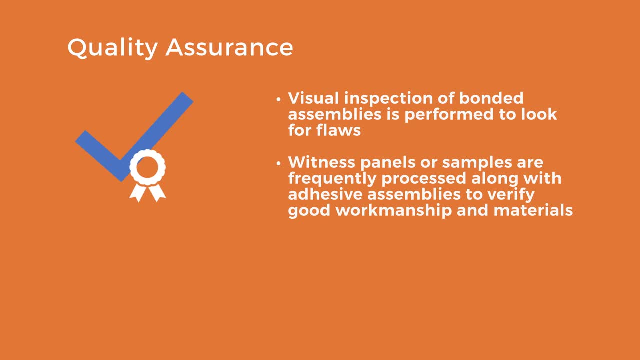 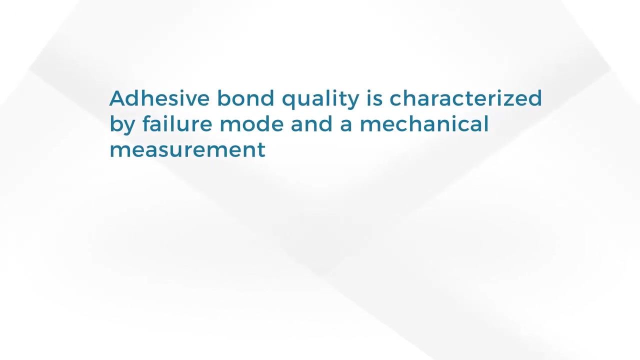 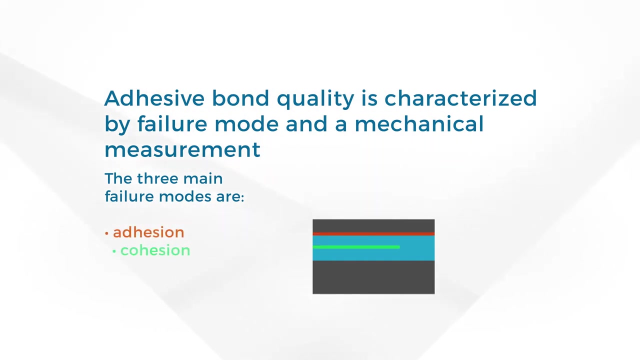 Witness panels or samples are frequently processed along with adhesive assemblies to verify good workmanship and materials. Various types of non-destructive evaluation are frequently used to verify the quality of adhesive bonds. Adhesive bond quality is characterized by failure mode and mechanical measurement. The three main failure modes are adhesion, cohesion and substrate interlaminar failure. 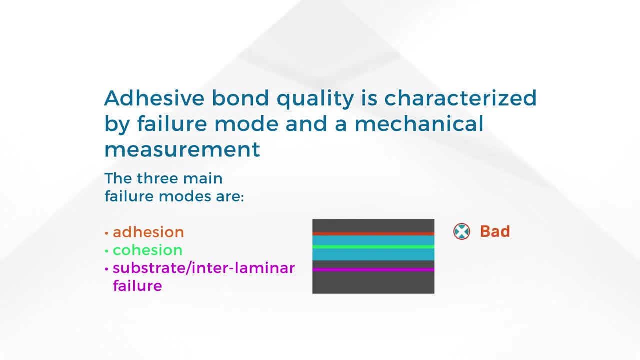 Adhesion failure mode is unmet. Adhesion failure mode is unmet. Adhesion failure mode is unmet. Adhesion failure mode is unacceptable, as this means the adhesive did not adhere to the adhering. Adhesion failure mode is unacceptable, as this means the adhesive did not adhere to the adhering. 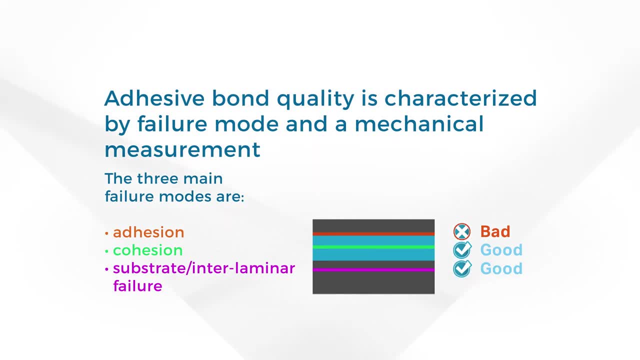 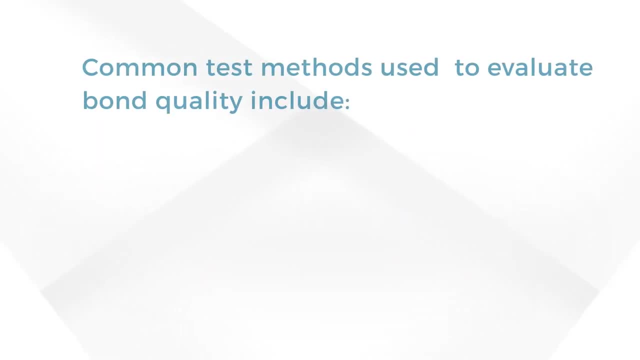 Cohesion. failure of the adhesive or substrate failure are acceptable failure modes as one can design to the mechanical properties such as fracture toughness of the adhesive and substrate respectively. Common test methods used to evaluate bond quality include lap shear, double cantilever beam.